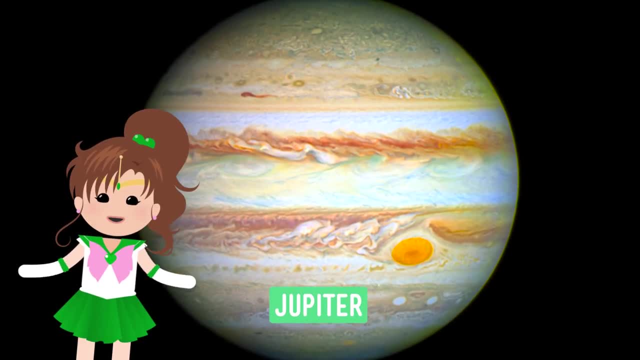 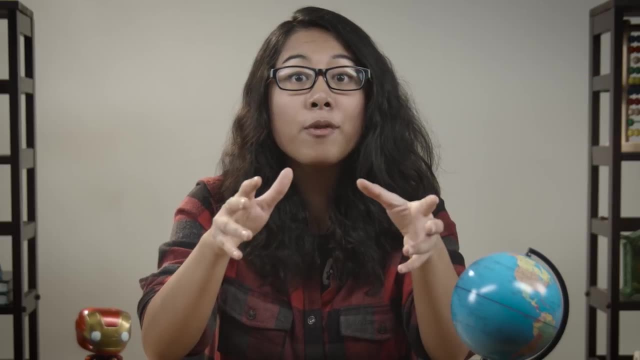 Jupiter is a big planet and its weather is equally big. It doesn't just have storms, it has STORMS. That's because the planet is surrounded by jet streams or fast-moving winds, some of which are flowing in different directions. When these opposing air flows meet, they create big, long-lasting swirling storms, Storms like the Giant Red Spot, a storm that's been brewing on the planet since possibly the 1600s- The 1600s, To make things even more interesting. the storm shrinks and grows in size and doesn't. 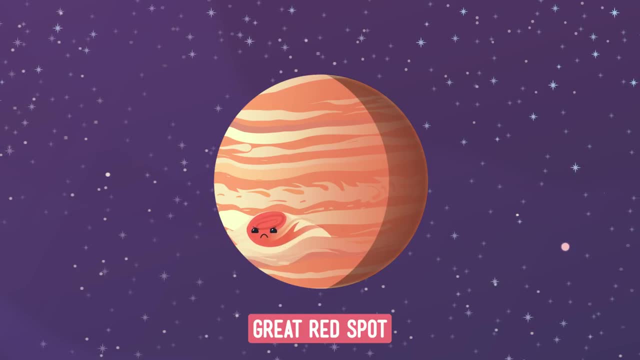 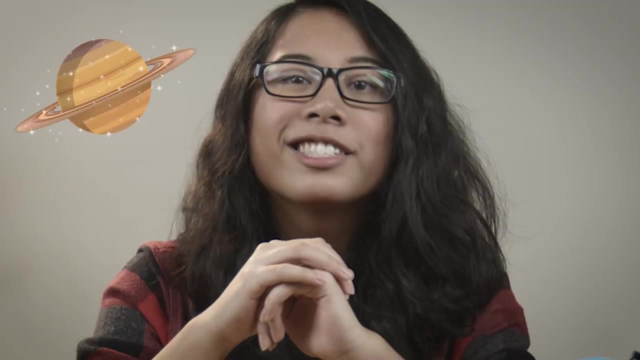 always stay in the same spot, although it always rotates in a counterclockwise direction below the planet's equator. And you thought storms on Earth could get wild. Let's take cover on our next planet, Saturn. Not that Saturn is less extreme. In fact, it's awfully windy here too. The winds on this planet can get up to 1,800 kilometers an hour. The strongest winds on Earth only get to about 400 kilometers an hour. These insanely fast Saturn winds, combined with heat from the planet's interior, are 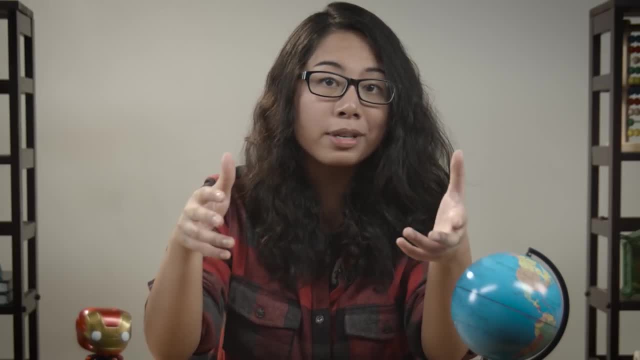 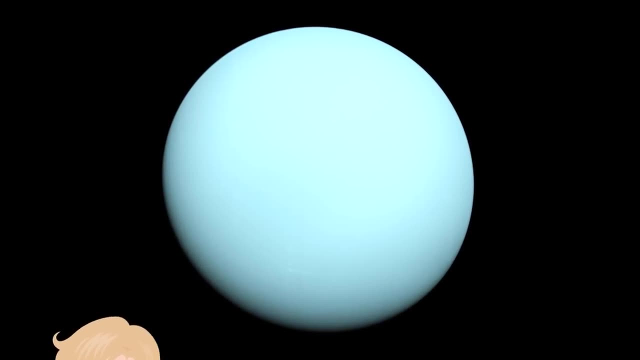 actually responsible for the yellow and gold bands we see in Saturn's surrounding atmosphere. So cold But pretty. Next stop, Uranus. Much like its gas giant neighbors, it's cold. The temperatures on Uranus can dip as low as negative 220 degrees Celsius. 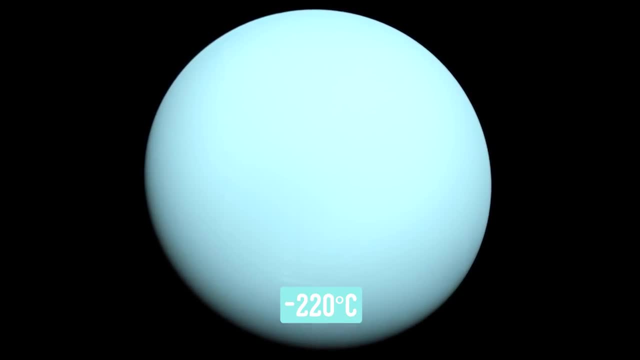 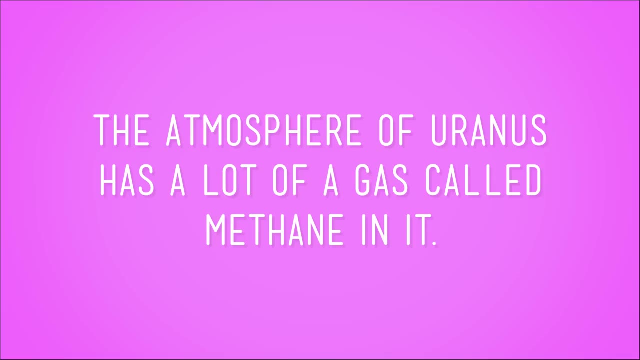 And, like Jupiter, it has pretty big storms, With winds almost as strong as those on Saturn. But it has one weird weather trait: Get this Diamond rain. How does that happen? Well, the atmosphere on Uranus has a lot of gas called methane in it. Methane is a greenhouse gas that explodes when you light it. The methane on Uranus is put under lots and lots of pressure, which splits the gas into carbon and hydrogen. The carbon is then compressed under all that pressure into diamonds, which are pulled down. 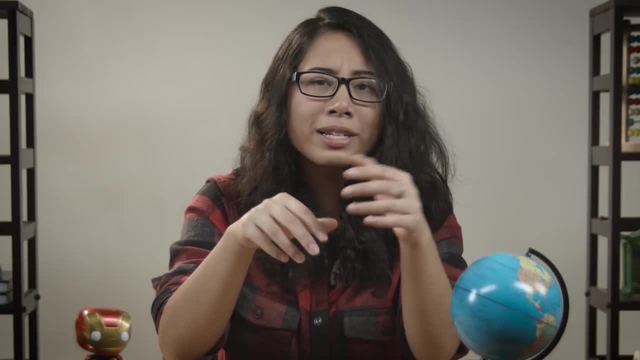 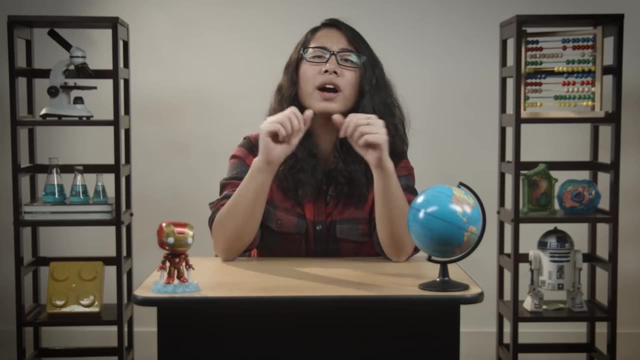 or rained down into the planet's core. So if you ever need to get rich quick, head down to Uranus And check out its diamond stash, You know. if you have the time to do a little space, travel On to our final gas giant, Neptune. Oh, what a surprise. Neptune also has extremely high winds, powerful storms and cold temperatures. I'm sensing a pattern here, But on Earth, the sunlight drives our weather. Neptune gets about a thousand times less sunlight than we do, So how do we explain its wild weather? 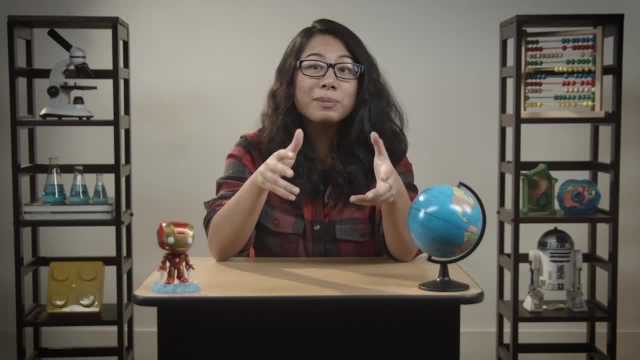 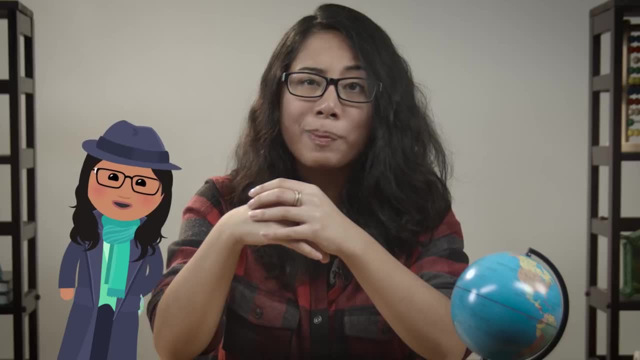 We don't, At least not yet. Scientists aren't sure how this planet gets the energy for its intense storms and winds, But we're not sure, We don't. We're just a little confused. I love a good mystery, Especially a good space mystery. So if you're traveling to the gas giants, brace yourself for crazy storms and winds on Jupiter, Saturn, Uranus and Neptune And maybe bring a big bag to stuff all those diamonds in. But keep in mind just like the rocky planets, the gas giants have weather sort of similar. 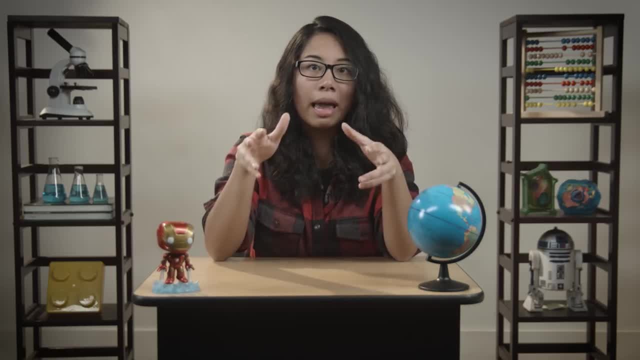 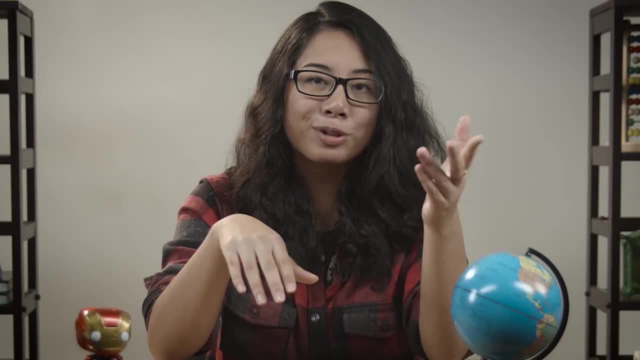 to what we have on Earth. Just you know, really amped up. I'm off to look for a warm, wind, free spot. I'm off to practice after school, to spend my afternoon and, just in case, maybe I'll keep my eyes peeled for diamonds falling. from the sky. You never know.